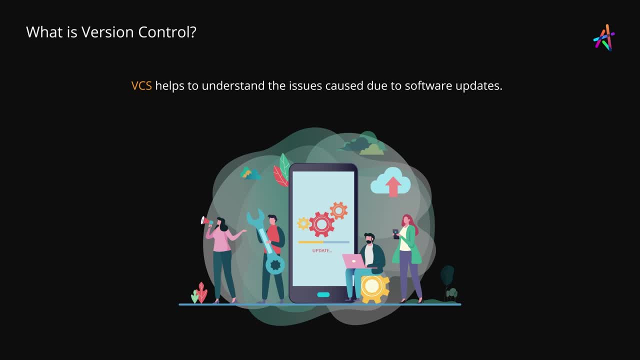 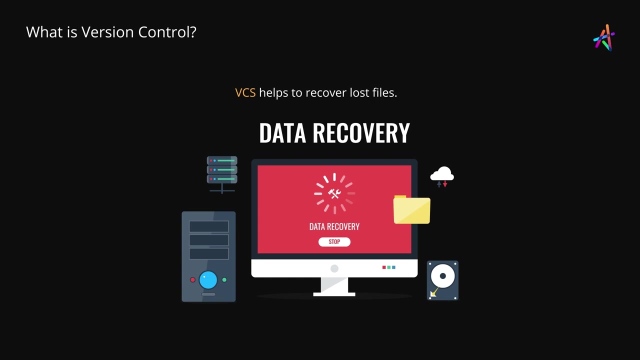 Well, we can use version control again. Version control helps you trace who last made the change and what is that change that could be causing that problem. We can also use version control to go back to the latest working version of that code And guess what All. 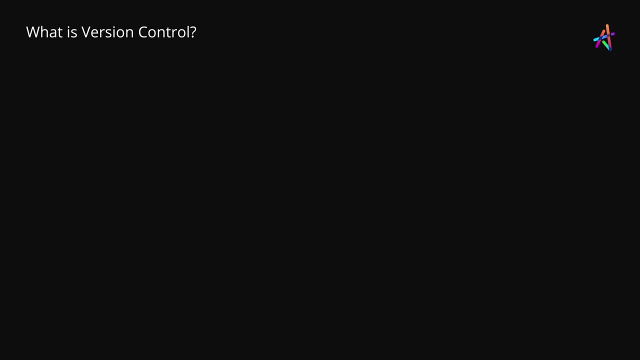 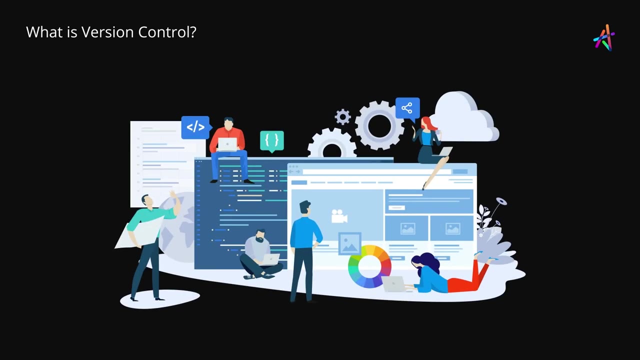 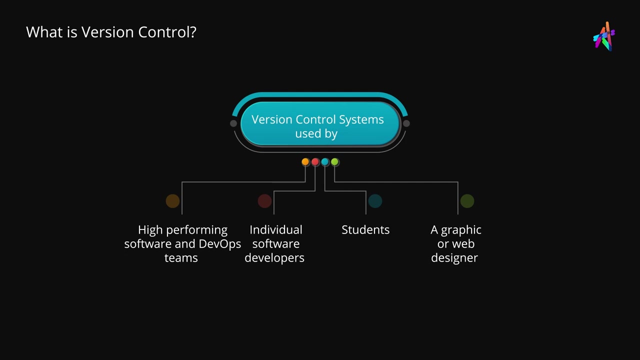 of this comes at a very little overhead. Who uses version control? Version control systems are an essential part of a modern developer's professional life. High-performing software and devops teams use it as a best practice to manage their source code control. Individual software developers who understand. 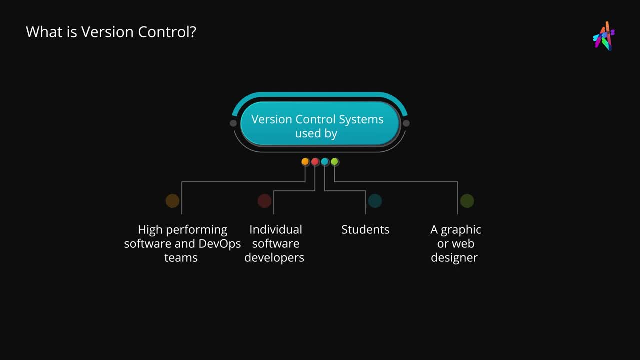 the benefits of a capable version control system, definitely need to ensure the proper system in their teams, typically use it even for their small solo projects or even for their non-software projects. Students could track versions of their notes or essays or even their project research papers. 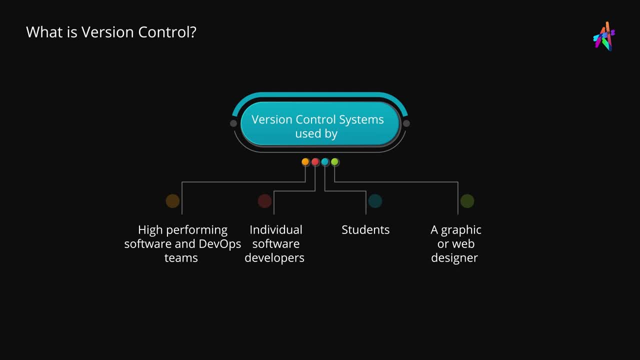 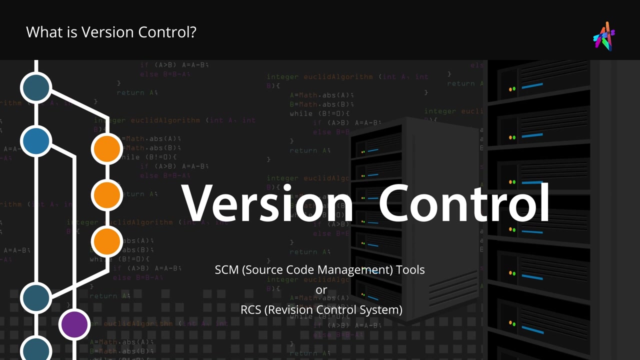 Graphic or web designers can use version control to iteratively modify different versions of an image or a layout without worrying about working or losing the only version of that image. Let's look at some of the popular VCS. Version control systems have evolved and improved to a great extent over the last few decades. 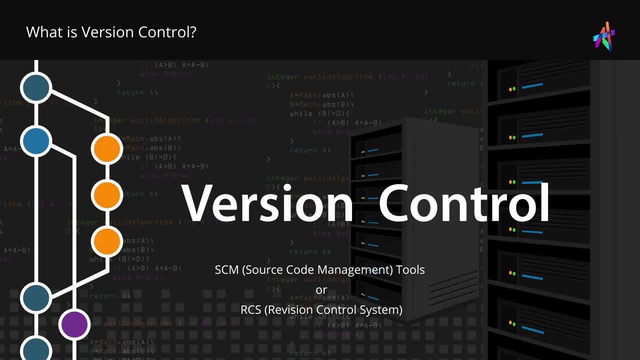 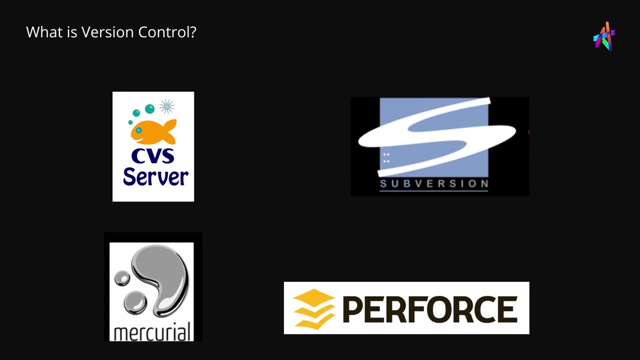 and some are better than others. VCS are sometimes even referred as SCM, Source Code Management or RCS Revision Control System tools. CVS, Subversion, Mercurial and Perforce were some of the popular VCS tools which have been the standard for version control for many years. 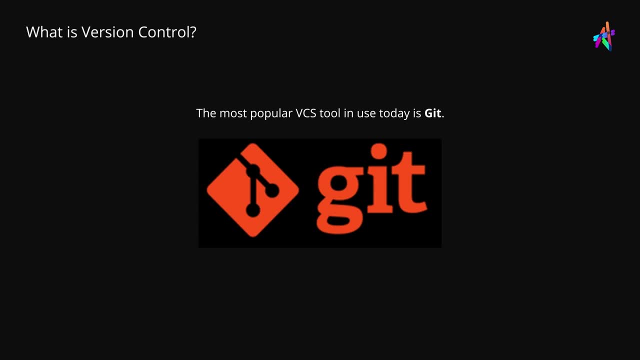 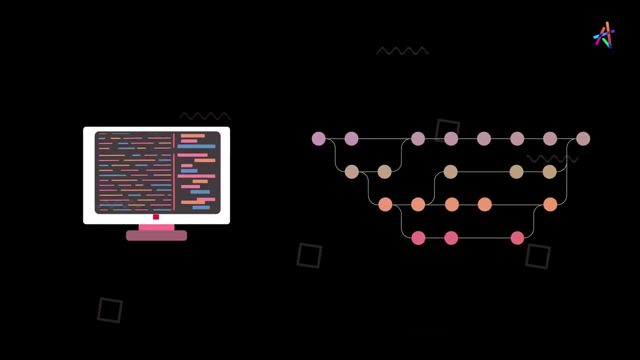 However, one of the most popular VCS tools in use today is Git. While it's possible to develop software without using any version control, doing so subjects the project to a huge risk that no professional team would be advised to accept. So the question is not whether to use it or not. 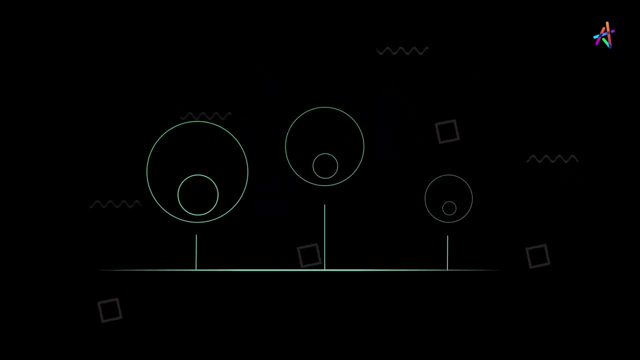 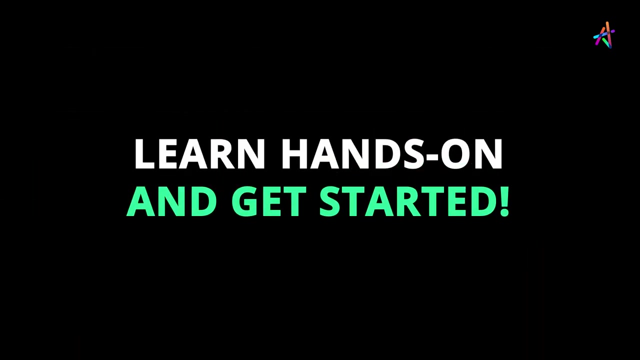 It's just a matter of time. So, which version control system to use? While there are many choices, the most widely used modern version control system in the world today is Git. Looking to leverage Git to enhance your workflow? Here's the perfect way to learn hands-on and get started.